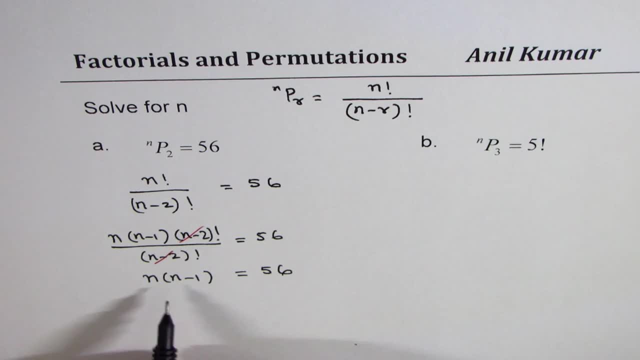 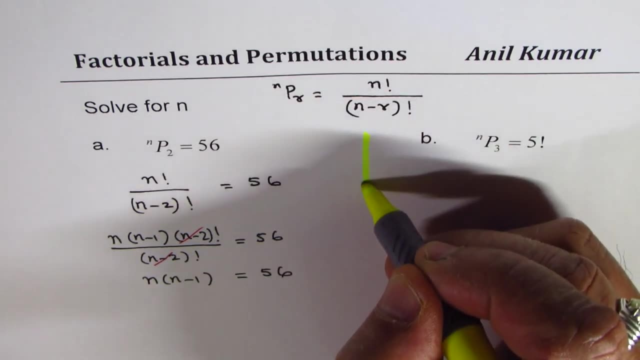 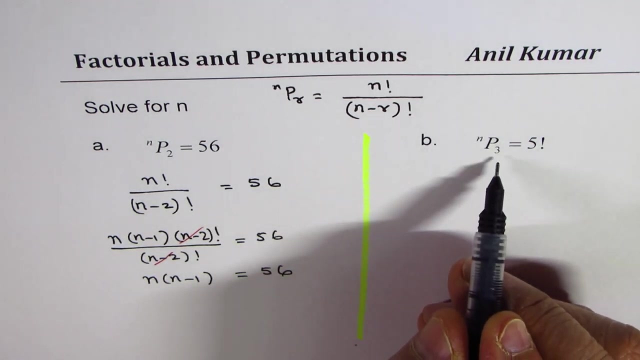 From here. this is a quadratic equation which can be solved and we can find the value of n. So you can actually pause the video. So we will solve this and find n. Let us look into the second one, which gives us: np3 equals to 5 factorial. 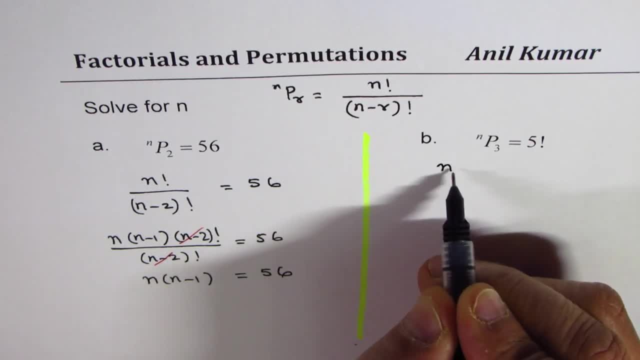 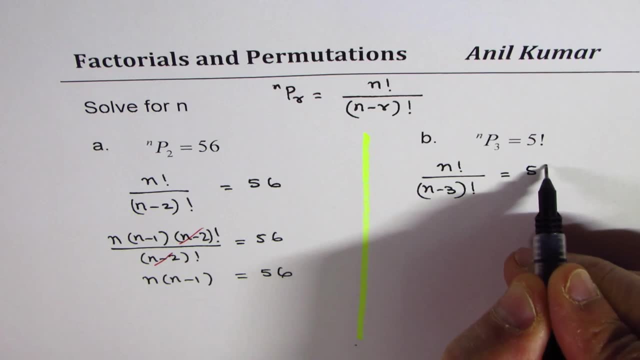 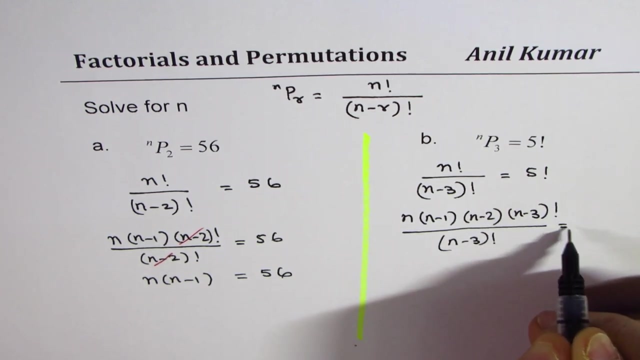 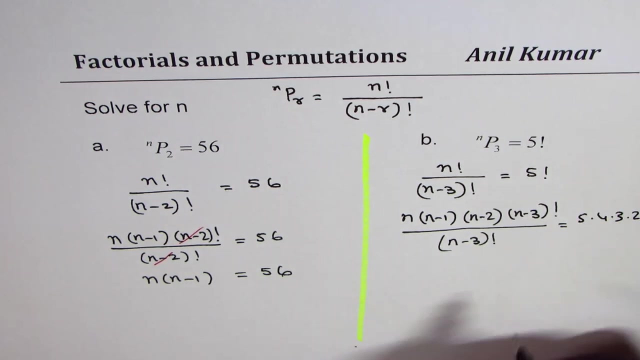 So I will continue with this. So that really means we have n factorial over n minus 3 factorial equals to 5 factorial. That means n times n minus 1 times n minus 2, times n minus 3 factorial divided by n minus 3 factorial equals to 5 factorial, which is, let's say, 5 times 4 times 3 times 2 times 1. 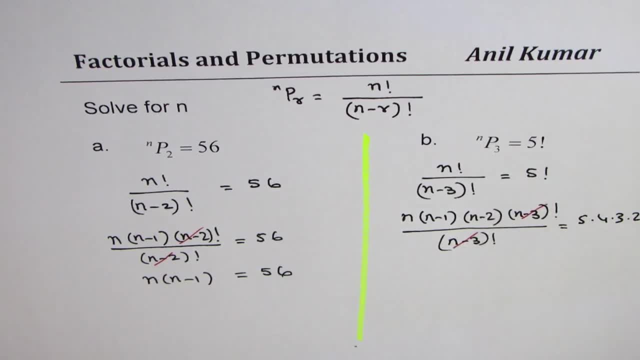 okay, now this and this cancels what really remains with us is a cubic equation: n minus 1 times n minus 2 equals to this number, which is 5 times 4 is 20 times 6 is 120. right, so that is what you. 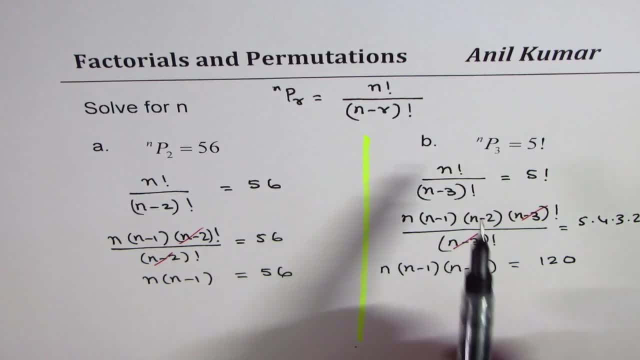 get and you get a cubic equation right. if i do np4 and something else, you will get a quartic equation. remember that. so so what really happens is that the r value in such questions may complicate your solution, depending on what the r is. if r is 5, you'll get degree 5 equation here to solve. 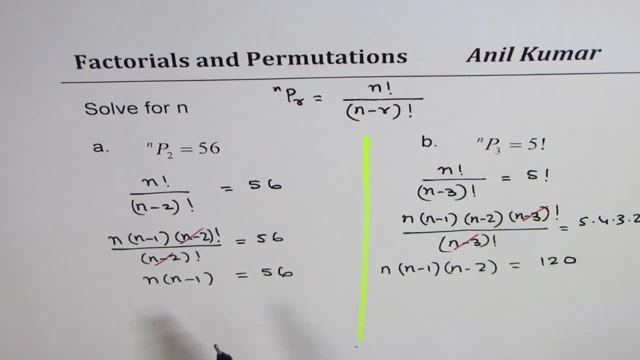 maybe in factored form. now the question is: how can i solve these equations quickly? right, i have to find the value of n. what i need to find is the value of n. this is what i need to find. how can i solve them quickly? now? the trick here is we could always solve them right. open the 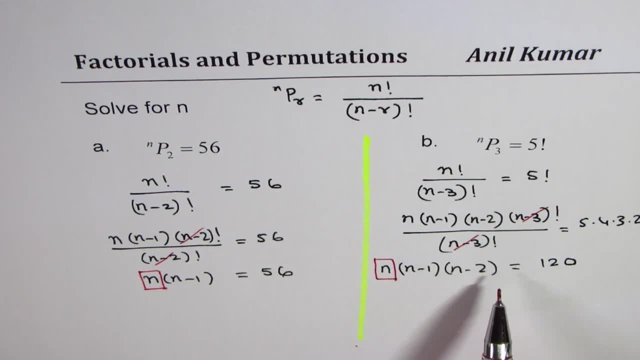 bracket, use the quadratic formula, factor out. you know it's a long process. how do we do it quickly? this is what i'm going to tell you in the next step. here it seems to be simple: 7 times 8, right, you have your answer right there. bigger number: you're looking for correct, uh, and here then what correct, so what? 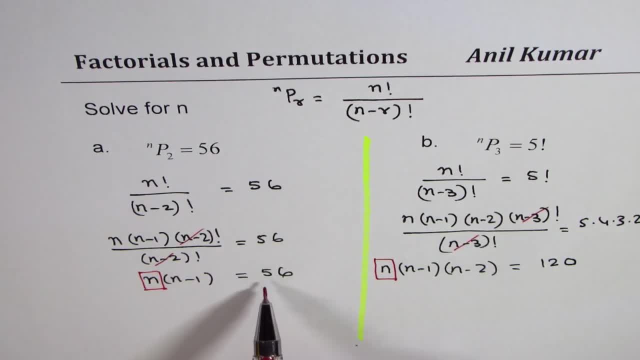 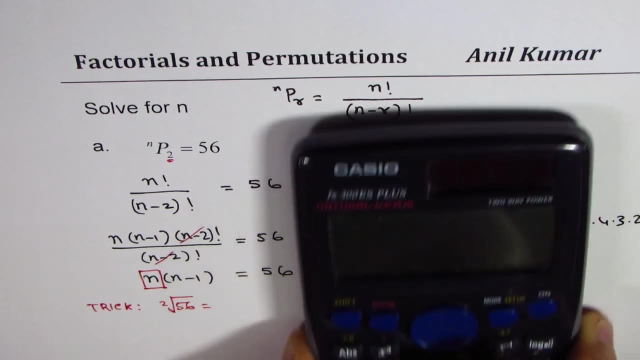 i do here is: if i have 2 here, we'll do square root of 56. so what we will do here is- i'm just discussing the trick here now. trick is: if this is 2, then we do 56 square root. what do we get? let's see so. so we have 56 and we- i'm 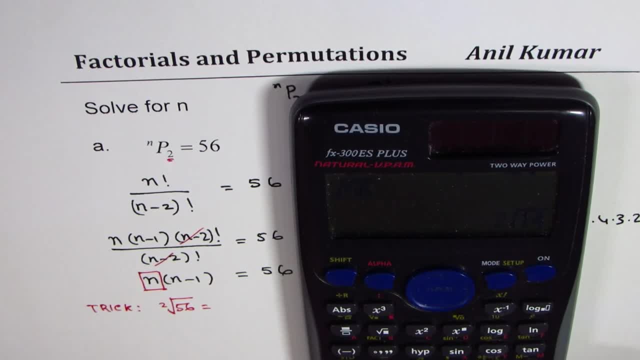 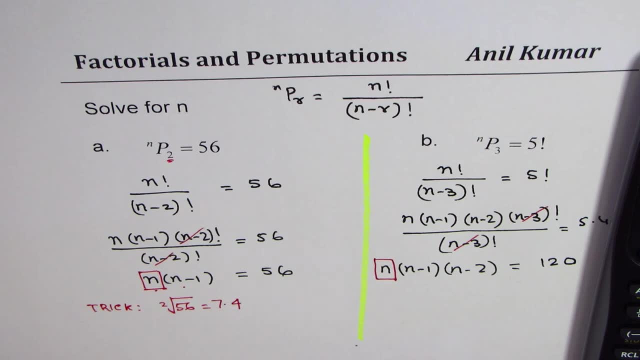 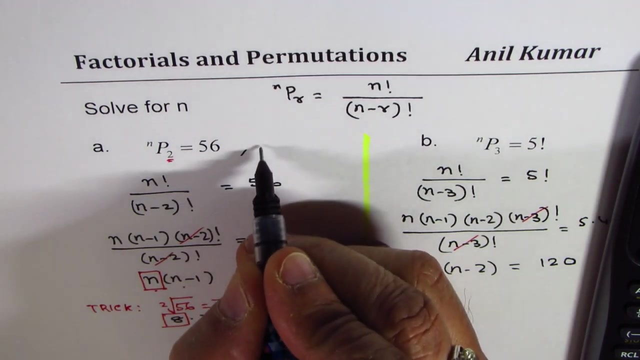 sorry, we do square root of 56 and we get in decimals 7.4. so we know these two numbers are around 7.4. so what are the possible numbers? obviously it is 8 times 7, 56, correct, and we get, and so we get our answer and that is: n should be eight, right, n should be eight. so we said that. 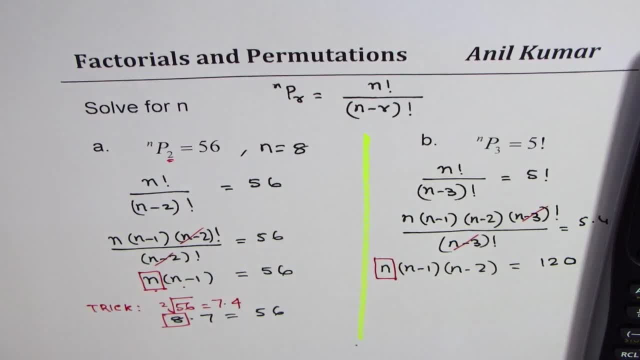 means n equals to eight. does it make sense to you? so what we have shown here is, without really solving the question, we estimated the square root right. you could estimate right. you know seven times seven is forty nine. we know seven square is forty nine and we know eight square is sixty four, like if. 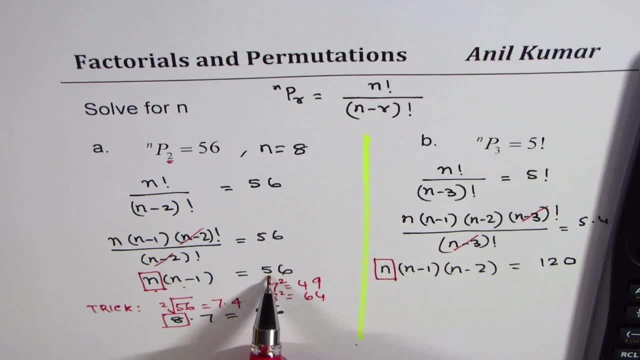 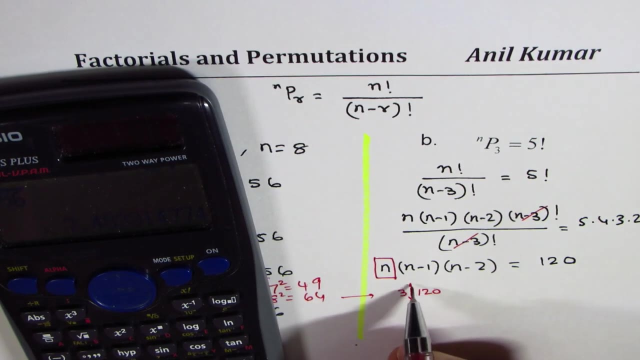 calculators are not allowed, then this number is in between these two and therefore we get our answer. you get my point correct. now we'll follow the same method here. so what i'm trying to do now here is we'll find the cube root of 120 and round it to a whole number. do you see that? so we have. 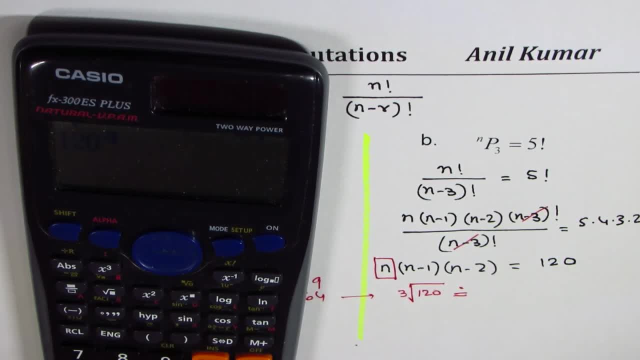 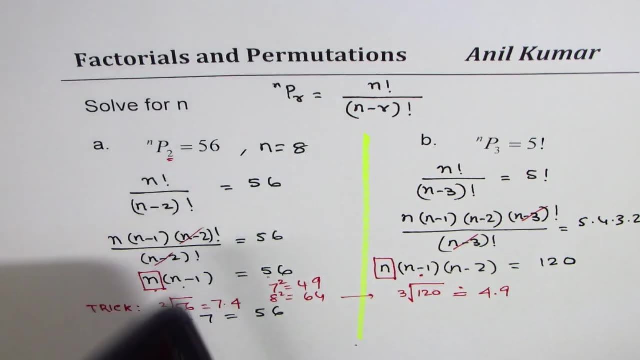 120 to the power of, let's say, 1 divided by 3. so that gives me the cube root right. so cube root of 120 is 4.9. approximately 4.9 is the cube root. that means the center value is 4.9, correct cube root. 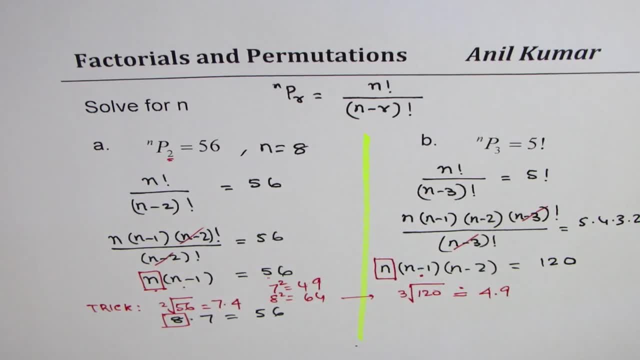 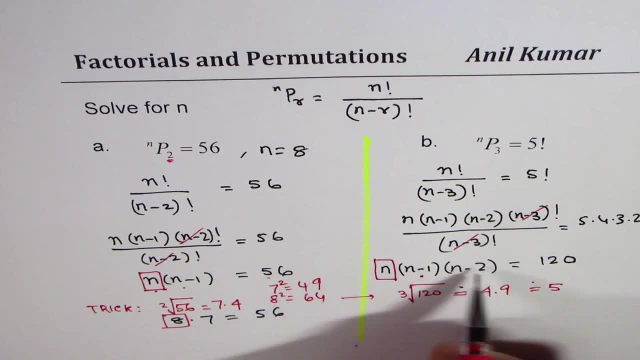 if you multiply three numbers is somewhere in between, do you understand? so the cube root is is approximately 5, 5, 5, therefore what the number should be. well, in that case, the center number is 5, these numbers should be 6 and 4 and therefore we get our answer as 6, and what you can do is you can perform a. 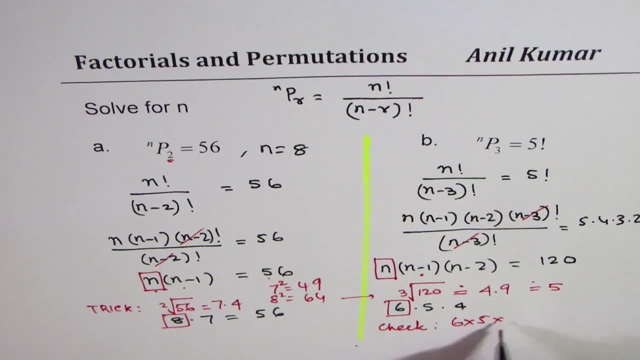 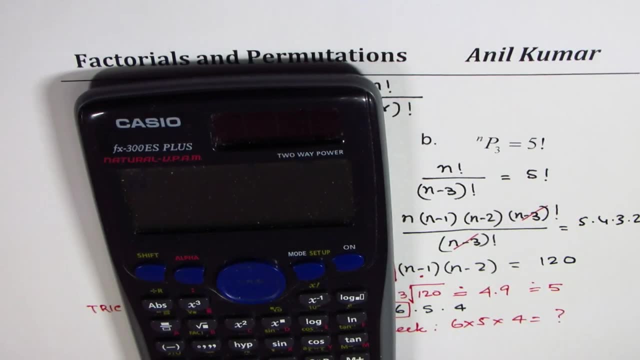 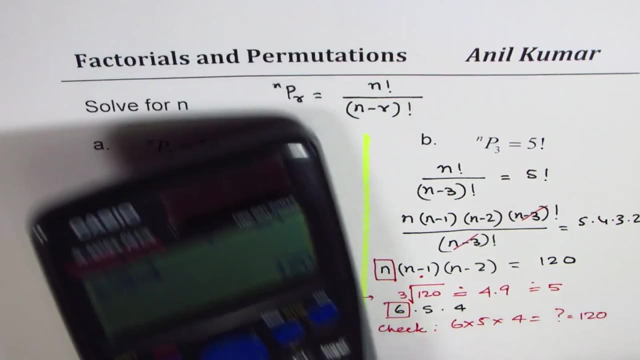 check. so what is the check? 6 times 5 times 4 equals to what? let's do it now. i know you could do it without calculator, but you know at times you could be working with degree 4 or 5, you could right. you get the same answer, 120, and therefore we can say n is. 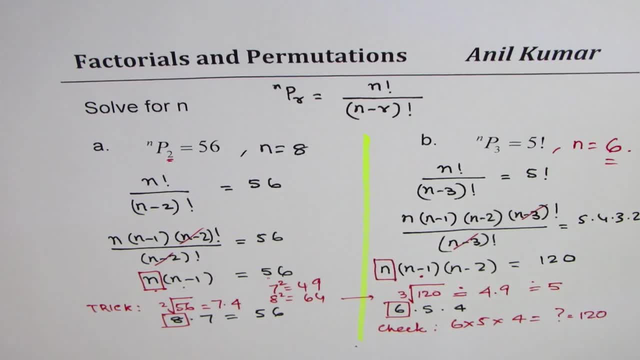 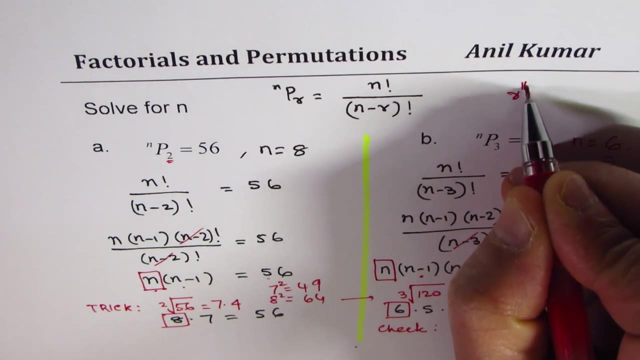 equal to 6. do you see that? so what i'm trying to emphasize here? that if you have multiple choice questions, restricted time and in general you could do nth root, i should say rth root- to get an answer in such a situation. i hope you're able to figure that out and i look forward to your questions and i look forward to your comments at the end of the week, this sort of of like practice. so we have a wholeשה nogle question text. it's not kali's case. you can dos here, so now again, let me do the same thing in this way, just to make sure you get the answer. we bed and 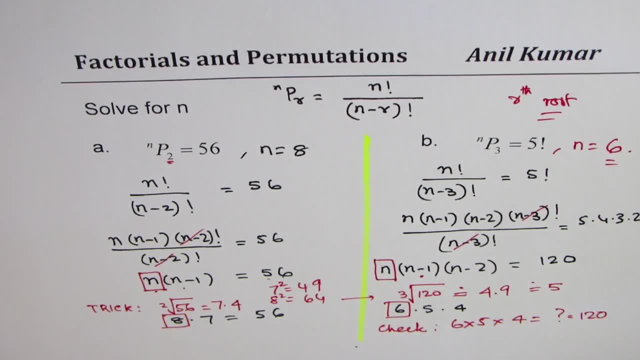 hundred wonders less questions you their class. okay, so it's 2018. I'm under treatment. how about that? did we give you a? you understand and appreciate this trick. that will really save time when really required. feel free to share my trick and my videos if you like. that'd be great. thank you and all the best. 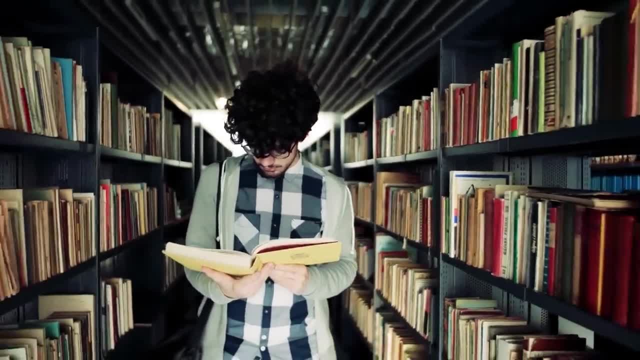 Everyone knows that the single best investment you can make in this world is in yourself. Personal development will help you blossom into the person you want to be, and it will help you stand on your own two feet. At a certain stage in life, we all reach that point where we want to start making money. 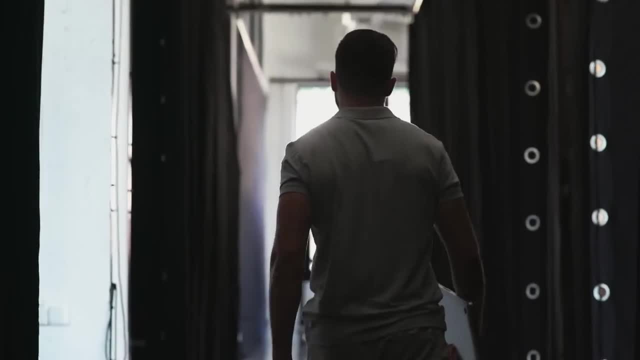 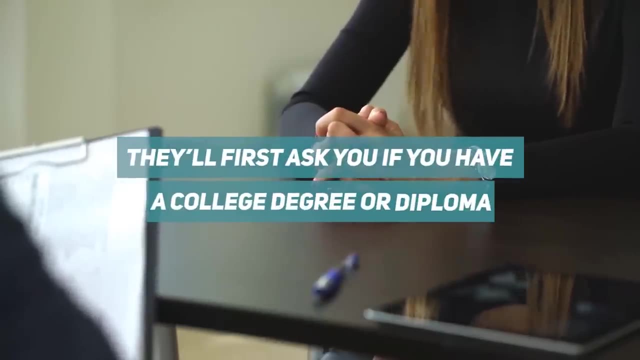 But the problem is you can't just walk into any random company and ask them to give you a job so you can make money. Chances are they'll first ask you if you have a college degree or diploma and if you do, they'll ask you: what value can you bring to the company? 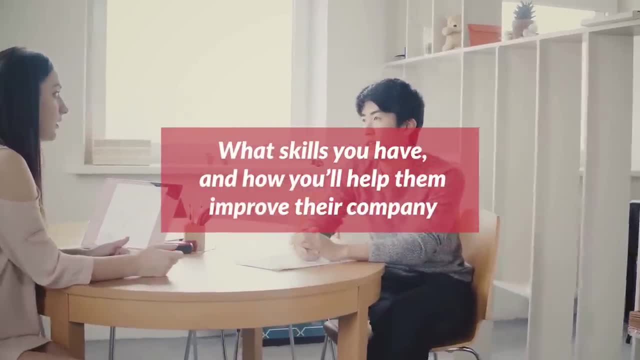 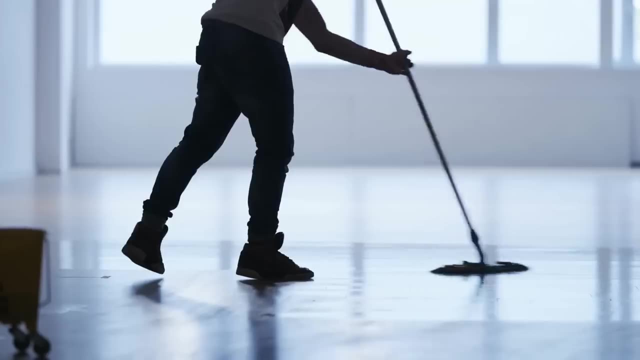 In short, they want to know what skills you have and how you'll help them improve their company In the marketplace. just about any skill will make you money, From cooking to cleaning, to cutting grass or hair, or to even accounting or marketing.